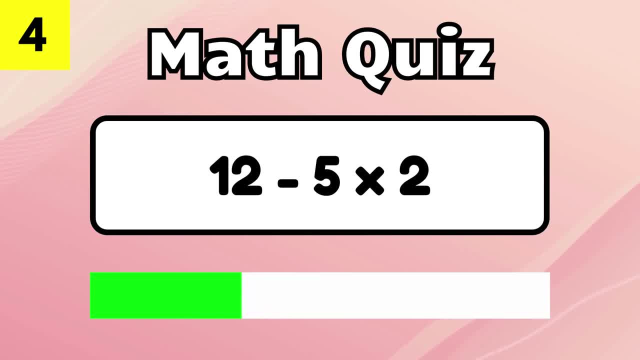 31, 32, 33, 34, 35, 36, 37, 38, 39, 40, 40, 41, 42, 43, 44, 45, 46, 47, 48, 49, 50, 51, 52, 53, 54, 55. 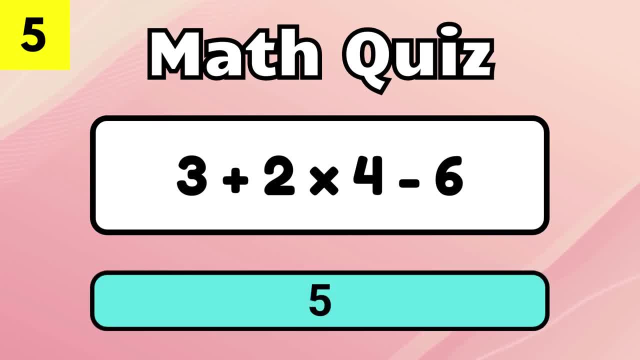 56, 57, 58, 59, 60, 61, 62, 63, 64, 65, 67, 68, 67, 68, 68, 69, 69, 69, 70, 71, 62, 63, 62, 63, 64, 65. 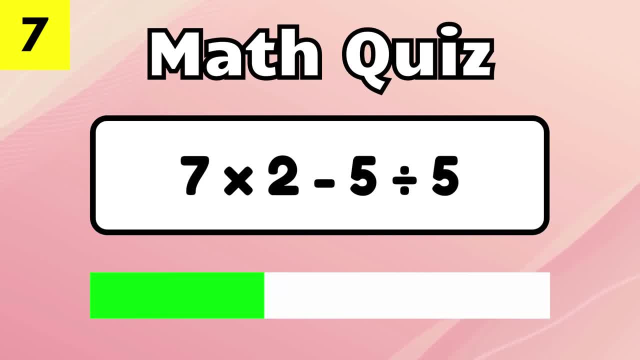 66, 66, 67, 67, 68, 67, 68, 69, 69, 70, 71, 72, 72, 73, 72, 73, 74, 74, 75, 76, 76, 77, 78, 78, 79, 80. 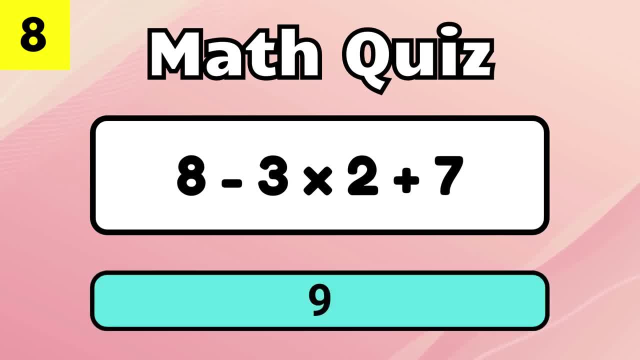 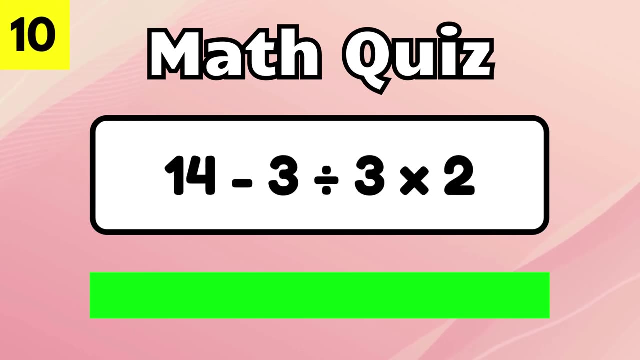 81, 82, 82, 83, 84, 85, 86, 86, 87, 88, 89, 90, 91, 92, 93, 93, 92, 93, 94, 95, 96, 97, 98, 98, 99, 100.